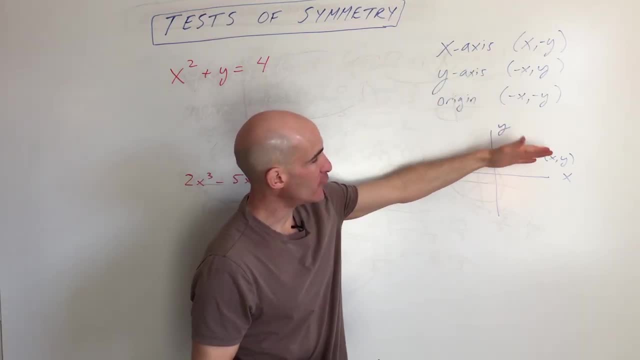 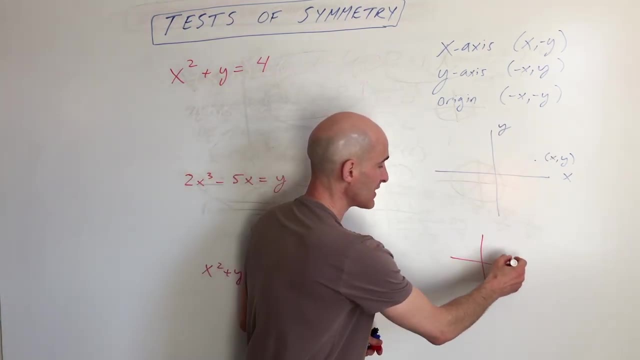 X-axis symmetry is that if you take the graph and you fold it over the x-axis, you reflect it over the x-axis, it will match up with itself. So for example, say for example, your graph looked like this: If you reflect it over the x-axis, it matches with itself. 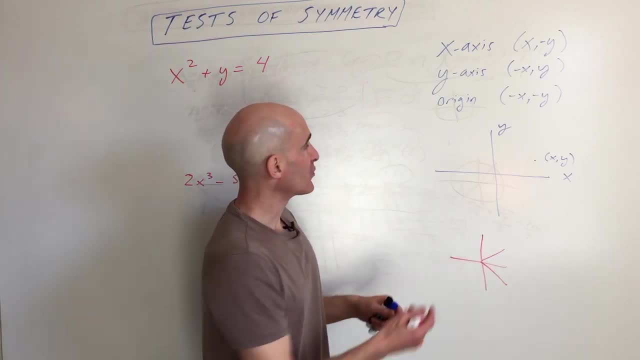 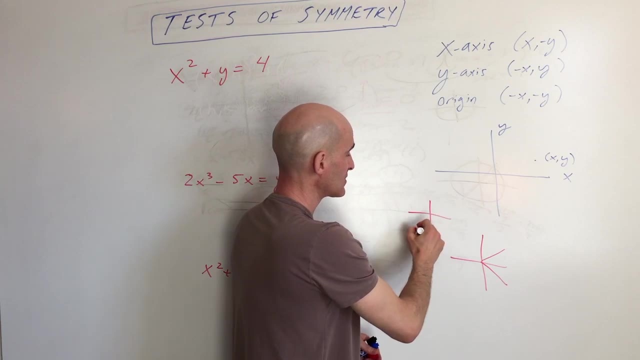 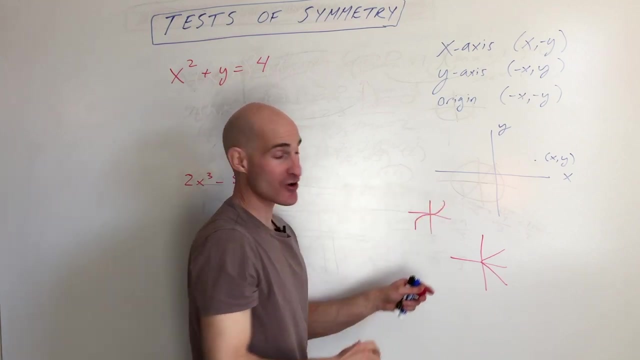 This is a line of symmetry of the x-axis. okay, Same thing with the y-axis. If you fold it over the y-axis, the graph will match with itself. And the origin is like this: For example, if you rotate it, you pivot it about that origin 180 degrees, like a half turn. it matches with itself. 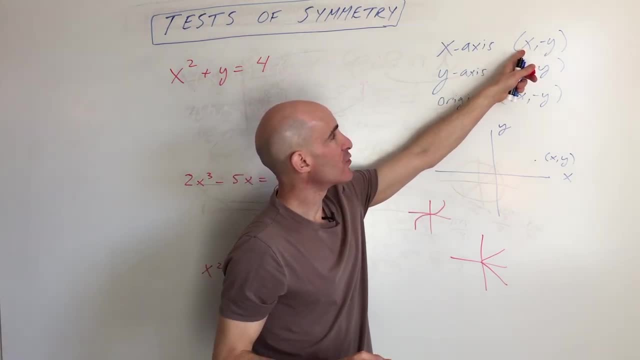 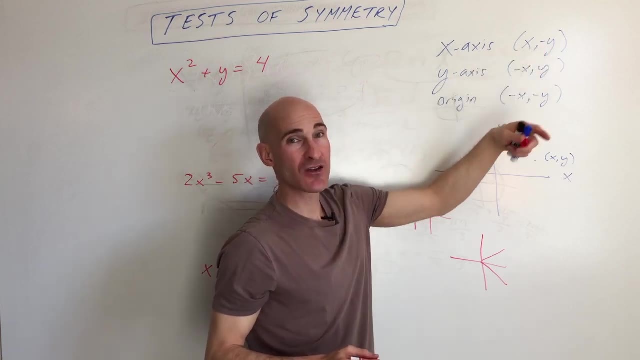 So these are the tests. So what you do is you replace in your equation x with x, y with negative y and then, when you simplify your expression, your equation, if you get back the original equation, that tells you that it has symmetry about that. 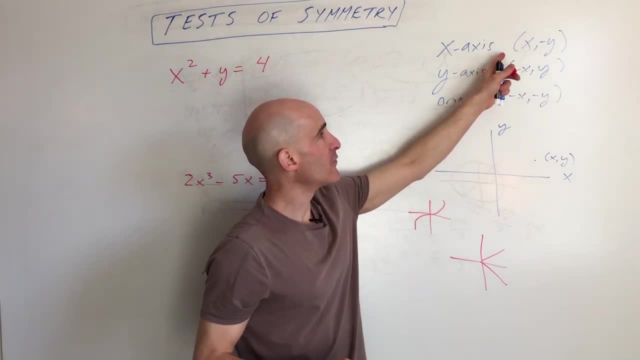 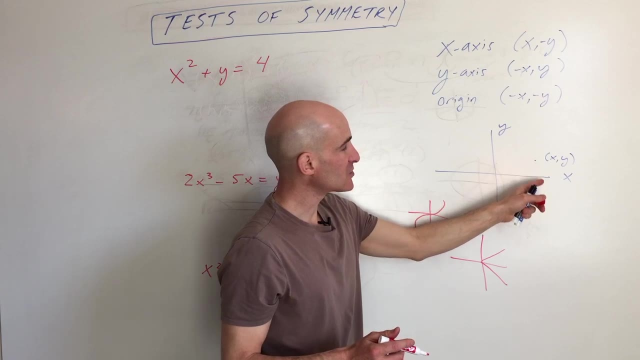 That axis or about that origin. So if you want to try to remember these a little bit easier, just go back to a simple point here in the first quadrant, x, y. If you reflect this over the x-axis, this point would be positive x, negative y. 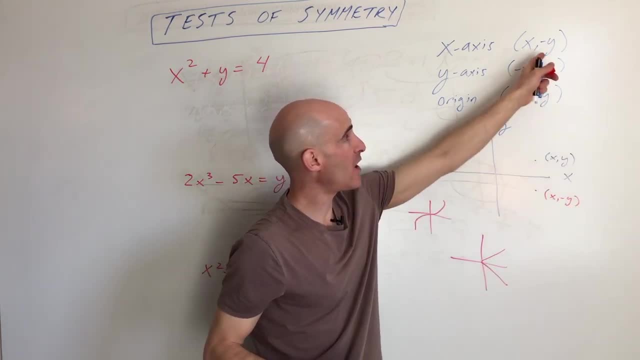 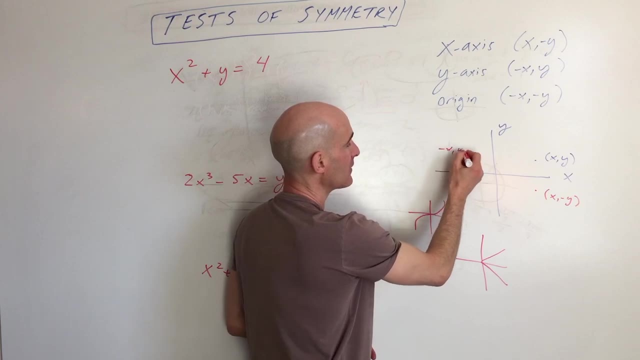 See, when you reflect it over the x-axis, this point will match up with x, negative y. and there you go. that's your test Y-axis. you're going to fold it over the y-axis, so you're going to be over here. negative x, positive y. 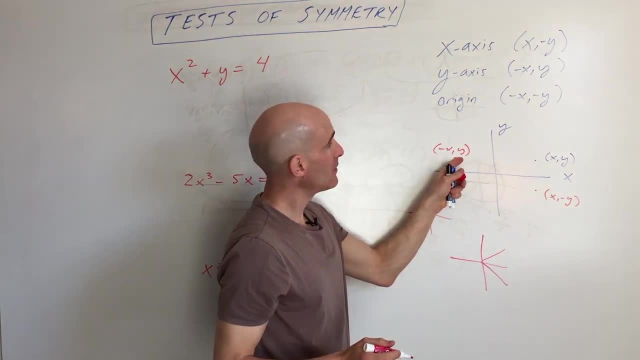 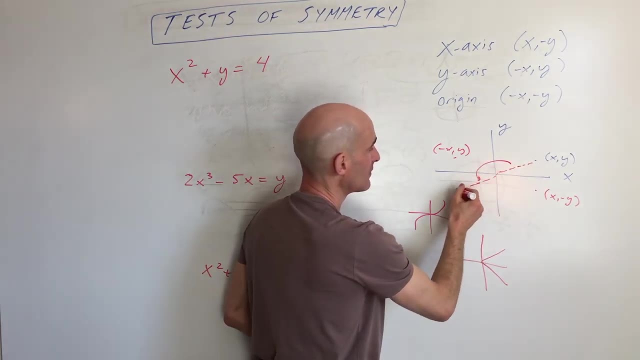 because you're going to the left, So you're going to be over here. negative x, but up the same amount. Okay, so that's your y-axis test and the origin. you're actually pivoting 180 degrees like this, and so now this point is going to be at negative x, negative y. 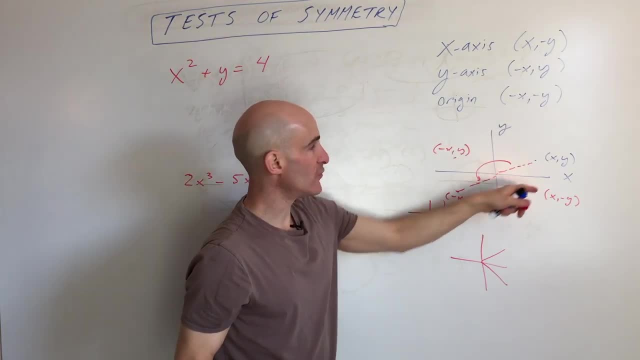 Okay, and that's the test for rotation about the origin. So if you want an easy way to remember, just go back to your coordinate axis system, pick a simple point here and look at what happens when you reflect it over the x, the y, or rotate about the origin 180 degrees. 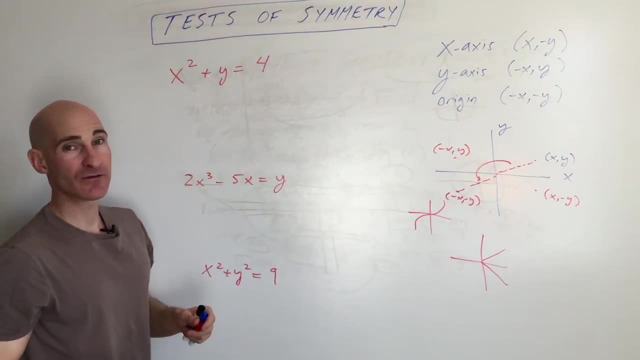 So let's take a look at a couple And let's see if we can test for the different types of symmetry that this graph may or may not have. So let's take that first one: x negative y. If we substitute x with x, we're going to get x squared, y with negative y. 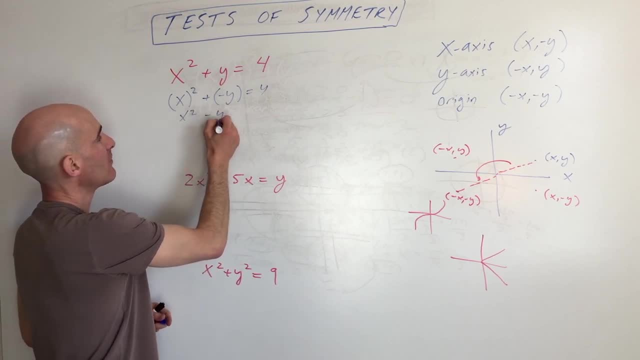 Okay, now when we simplify, you can see this is just going to be: x squared minus y equals 4.. Does this look like the original equation? Nope, it's a little bit different because of the negative y. Okay, so you can see that. 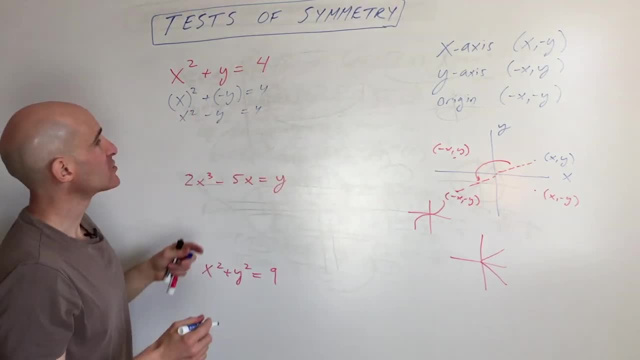 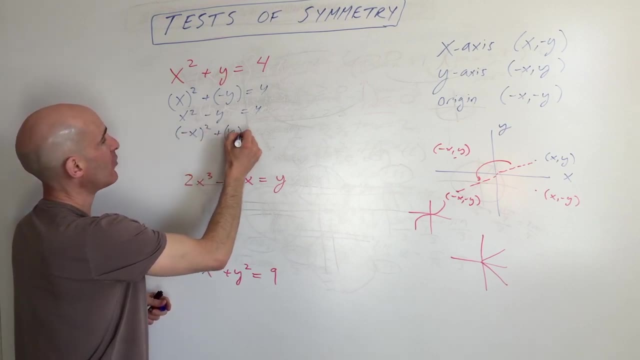 Okay, Okay, Okay, Okay, Okay. This does not have x-axis symmetry. Let's do y-axis symmetry now. So now we're going to replace x with negative x, y with positive. y equals 4.. So usually when I do a substitution, I put it in parentheses, so it's taken as a group or as a whole. 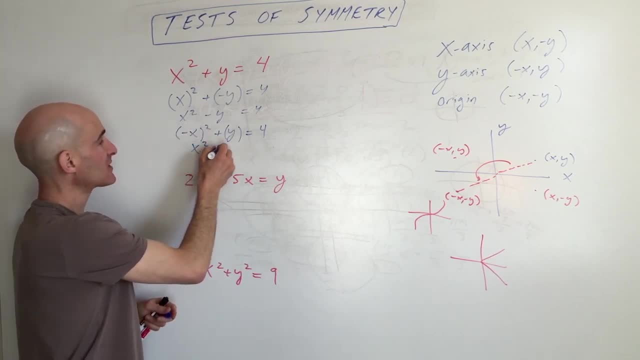 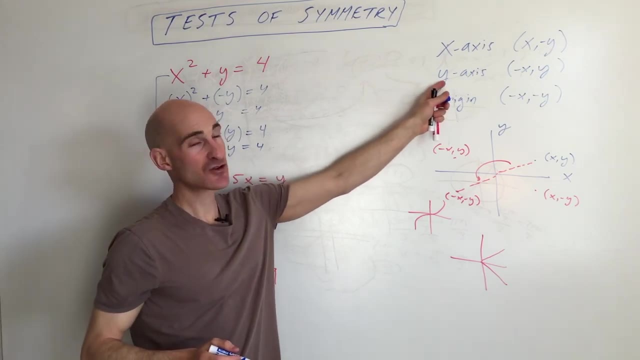 A negative to an even power is positive. So this is going to be: x squared plus y equals 4.. We have a match that tells us that it's symmetric about the y-axis. Okay, If you fold it over the y-axis, it will match with itself. 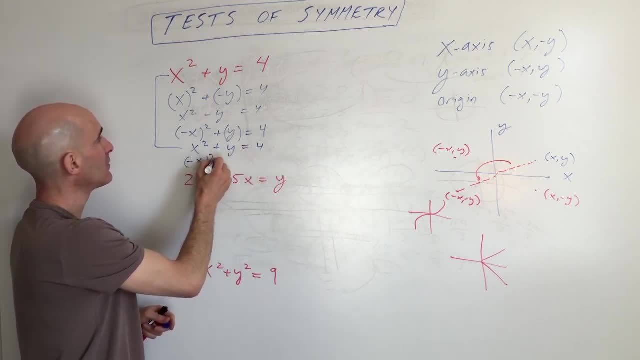 And then the last one, the origin. we're going to make them both negative, And if you simplify this, you get: x squared minus y equals 4, which again does not match the original one. So in this case you just have y-axis symmetry. 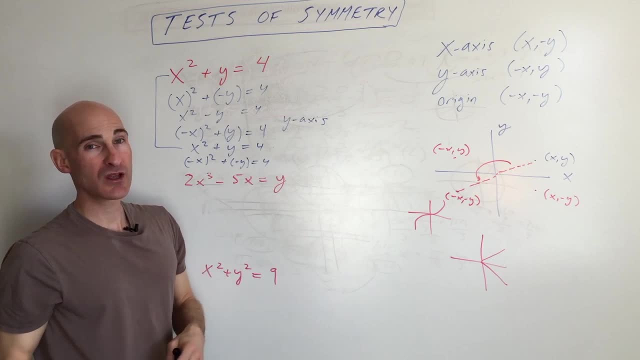 I want to let you know. it could have more than one, It could have two, It could have all three, It could just have none. So you just have to test them and see. So let's look at the next example. 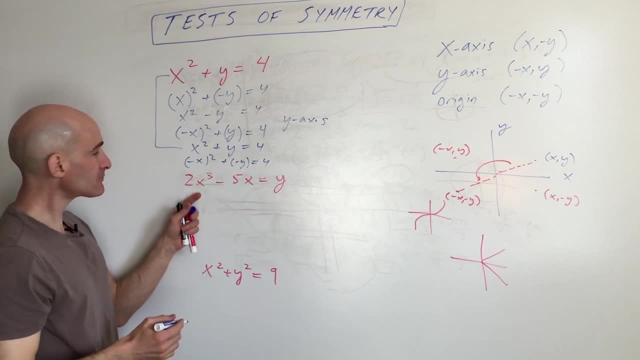 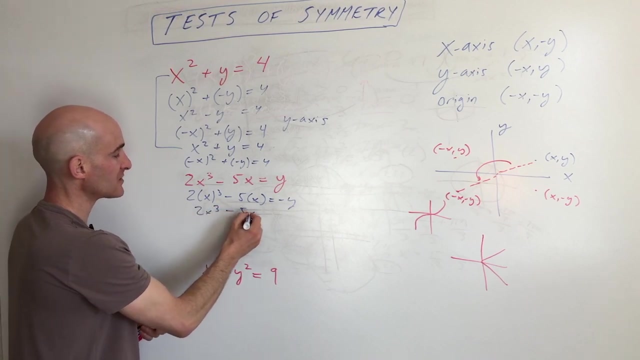 This one. here we've got 2x cubed minus 5x equals y. Let's replace x with x and y with negative y. So that's going to be okay. if we simplify, we get 2x cubed minus 5x equals negative y. 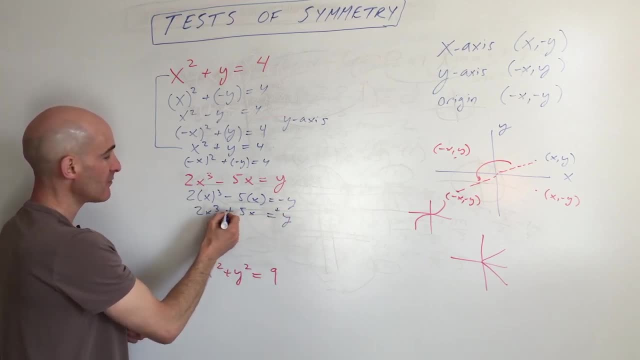 Even if we multiply everything by negative 1, this would be positive, positive and negative. Okay, Multiply everything by negative 1.. Still, it doesn't look like the original equation, So It doesn't have x-axis symmetry, y-axis symmetry. we're going to replace x with negative x. 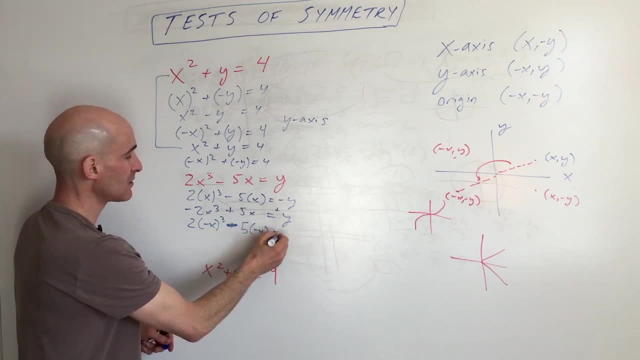 Oops, that's a minus right there. minus. Okay. If we simplify this, we get negative 2x cubed positive 5x equals y. Here you can see the signs are again not the same, So it doesn't have a y-axis symmetry. 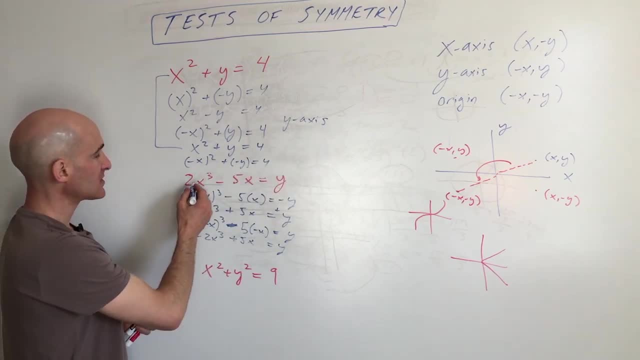 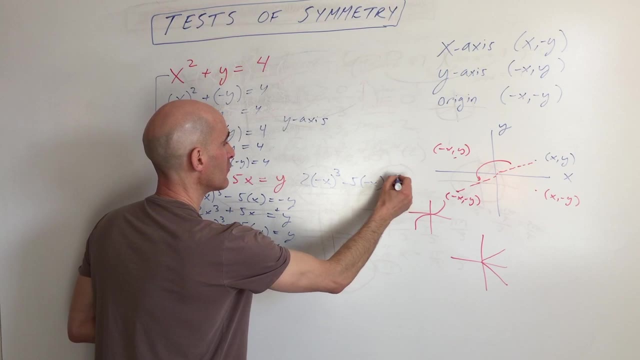 And the last one, origin symmetry. we're going to replace x with negative x, Okay, y with negative y, And if we simplify we get a negative 2x. cubed plus 5x equals negative y. If we multiply everything by negative 1, we're doing it to both sides. 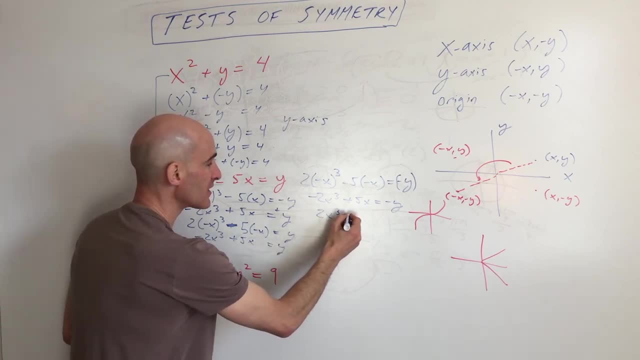 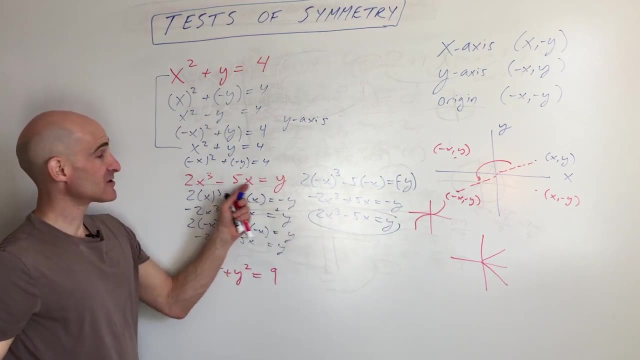 We're not changing the equation, but we do change the way that it looks slightly here. Now look what we have here. We have a match. Okay, These are exactly the same. That tells us that this graph is symmetric about the origin. 180-degree rotation about the origin. 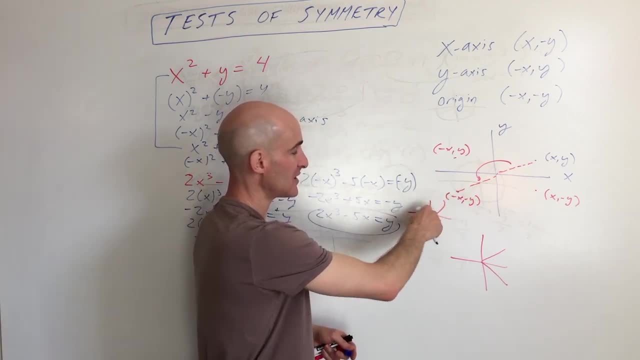 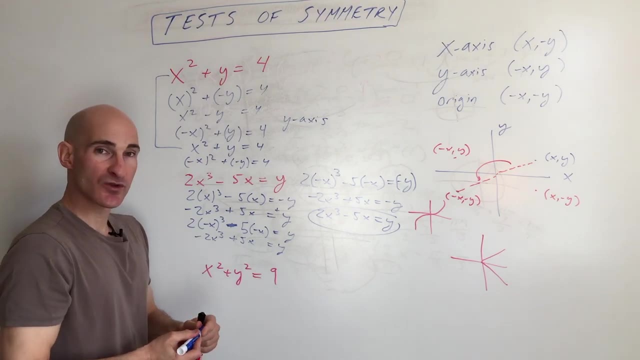 It will match with itself, similar to a graph like this where you rotate it, you're pivoting about the origin and it matches with itself. Last one here: x squared plus y squared equals 9.. So this one here. we're going to do this a little bit more intuitively this time. 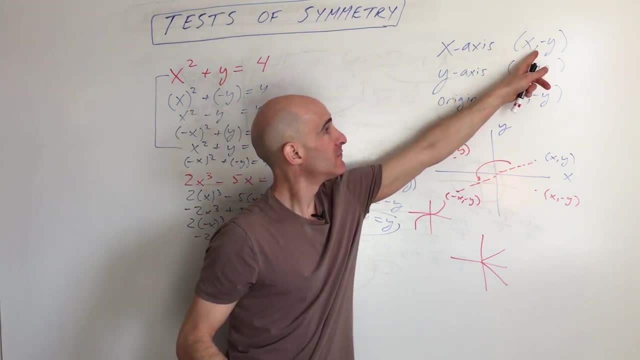 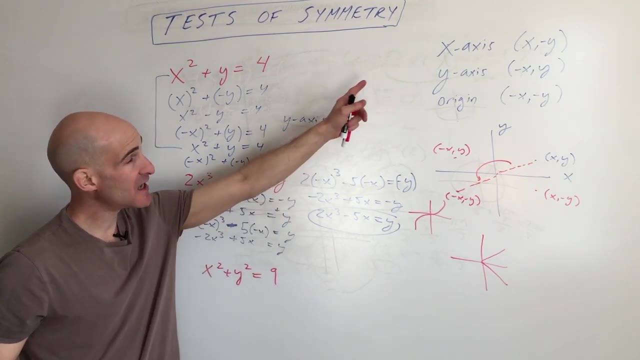 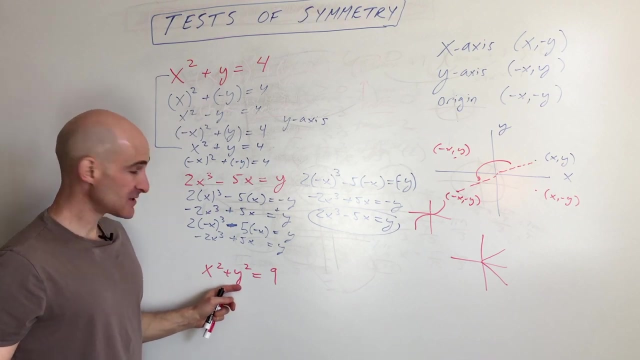 If we replace y with negative y, a negative squared is still a positive. So you can see we're going to get back to the original equation. So it does have symmetry about the x-axis, Same thing with y-axis symmetry. If we replace x with negative x and y with positive y, a negative x squared is positive x squared. 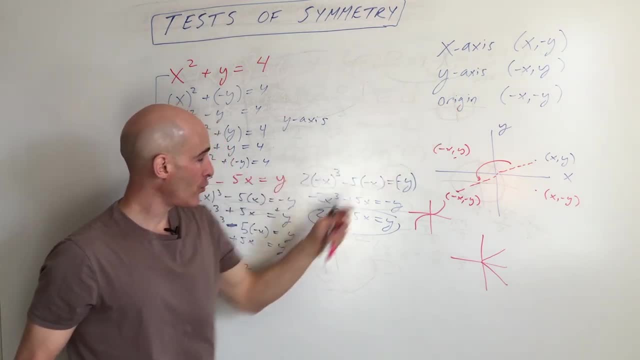 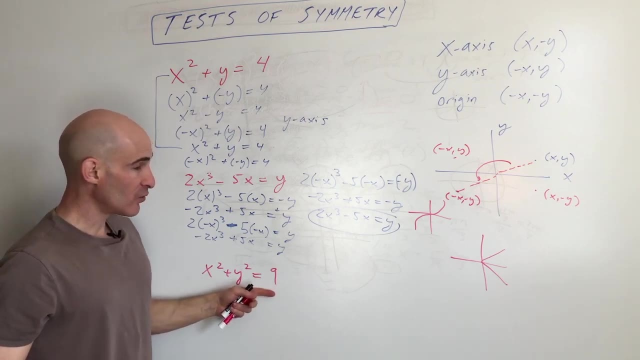 We're going to get back to the same equation. Okay, good. And then origin. if we make both the x and the y negative, still these are raised to even powers. They're going to be positive. This equation will be the same. 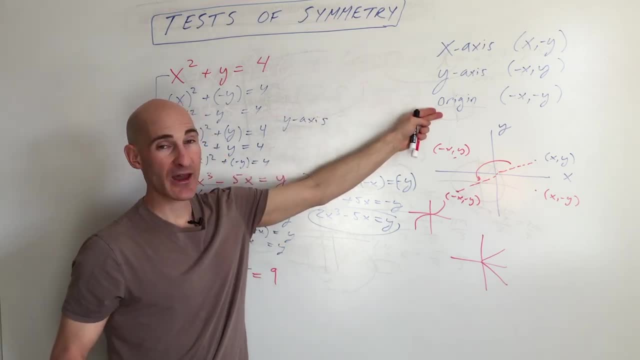 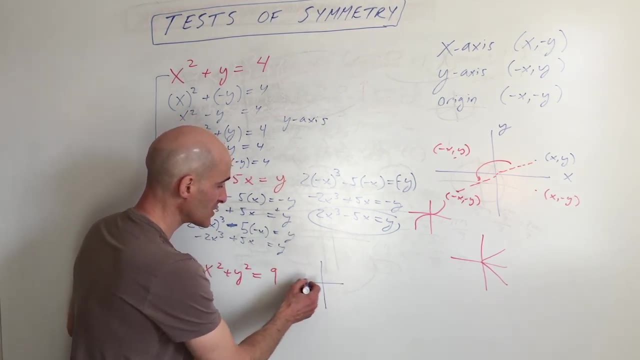 So what this tells you? it actually has symmetry about the x-axis, y-axis and the origin, And we know this from a previous video about circles. This is just the equation of a circle with radius 3.. The square root of 9 is 3.. 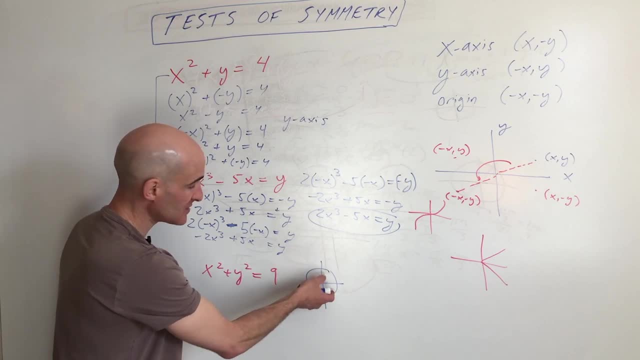 And we know that if you fold it over the y-axis, fold it over the x-axis or rotate it 180 degrees, this graph will match with itself. So this has been an overview about how to find the symmetry in graphs, given the equation, using these symmetry tests. 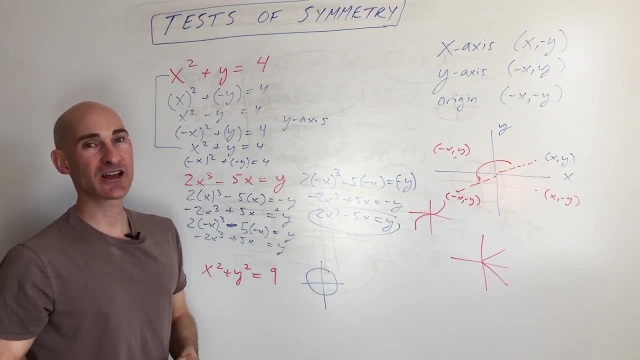 If you have any questions, review it again, take another look and I'll see you in the next video.